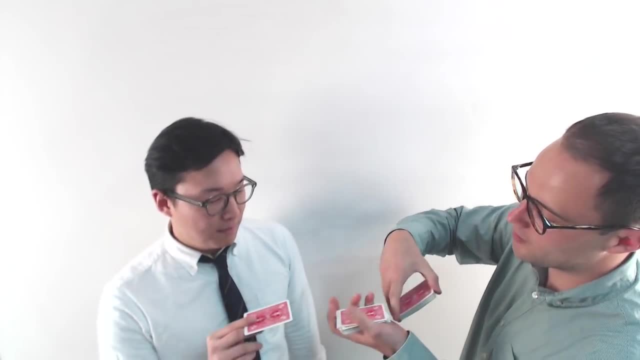 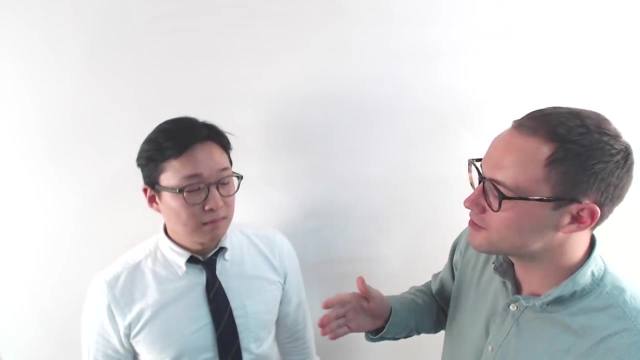 Sorry, Go ahead and tell me again when to stop. Stop, Okay, Puts it in there again. What would be the probability of him choosing the card again? What do you think, So getting a joker and a joker a second time? what do you think the probability? 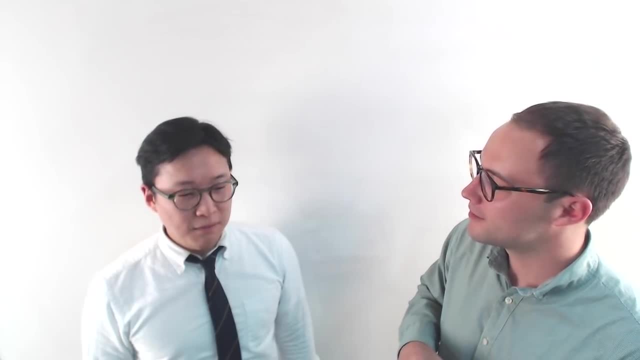 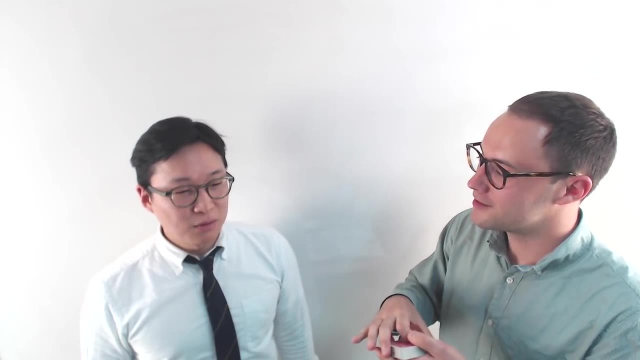 How many cards? So now we've got 54, total 54, then 154.. Okay, But there's actually two jokers still, Yeah, So two, Two out of 54.. So let's see if he can randomly choose it again. Ready, Tell me. 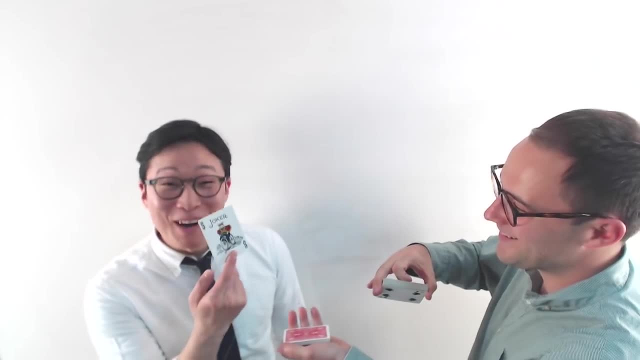 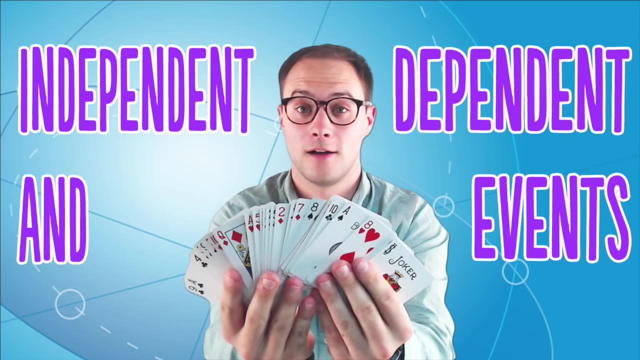 when to stop. Stop There, All right. Oh my god, And he got it again. So welcome to Anywhere Math. I'm Jeff Jacobson, This is Cal, And today we're going to talk about independent and dependent events. Let's get started. 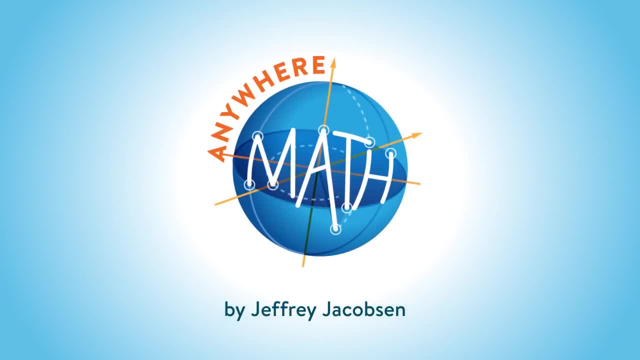 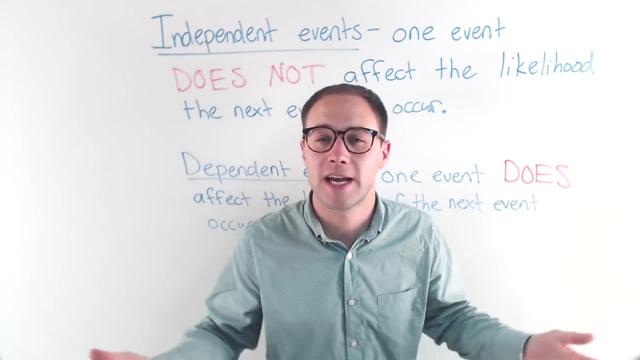 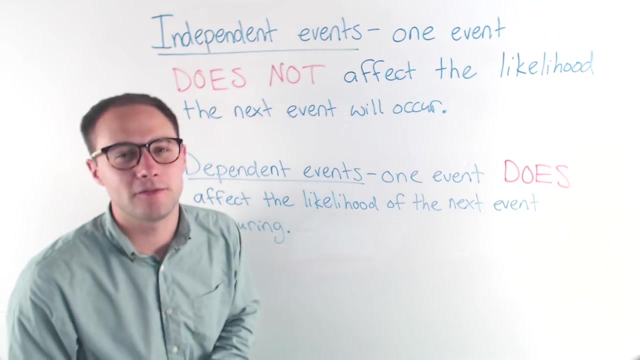 All right. So today we're talking about independent versus dependent events. So first let's talk about what exactly those are. We're talking about compounding Compound events. These are two types of compound events. So first, independent events are when one 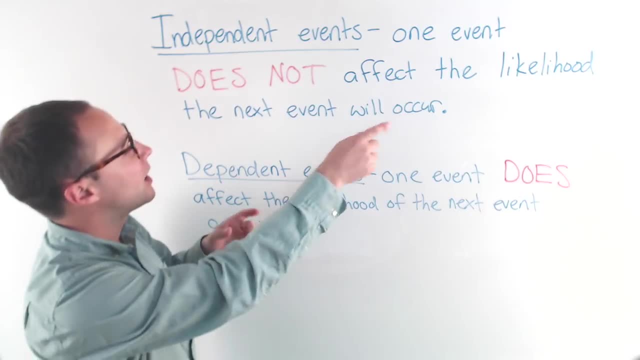 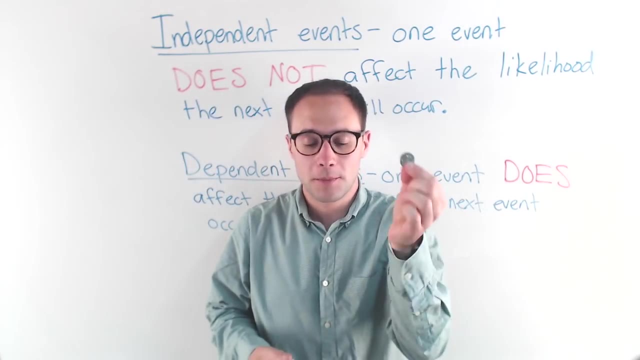 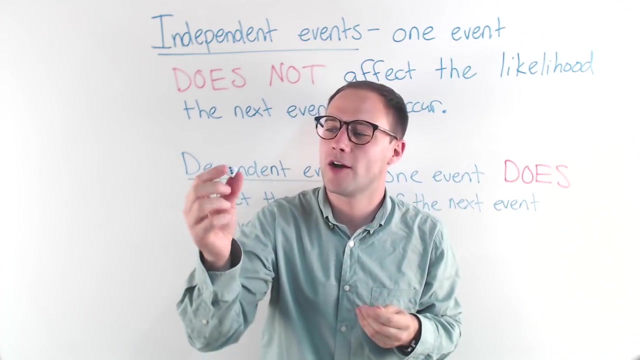 event does not affect the likelihood the next event will occur. So let's kind of talk about that in plain English. Let's say our two events were flipping a coin and rolling a die. Now, if I flip heads, does that change the probability of me rolling a five? No right, This die does not. 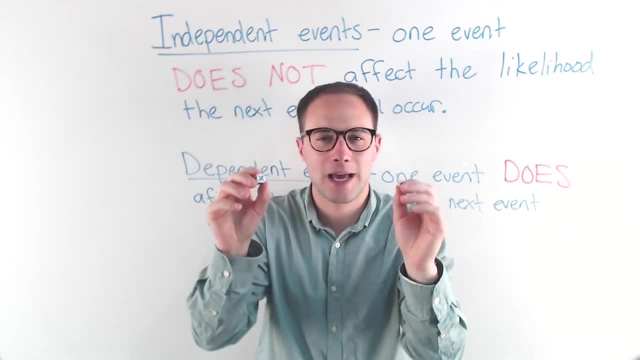 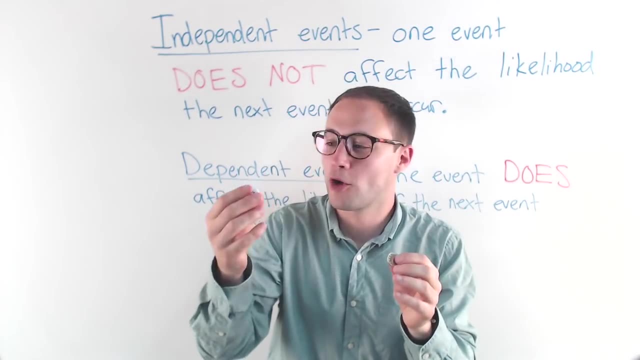 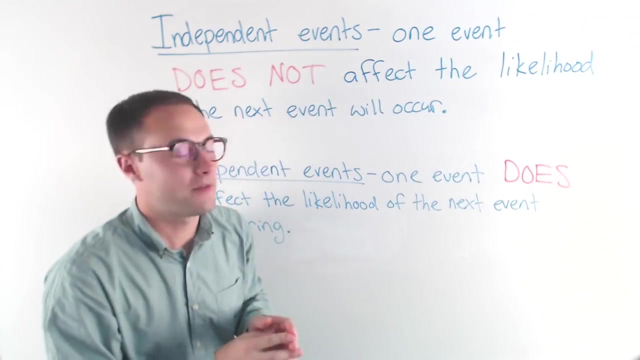 care What I flip here. these are completely separate. They are independent of one another. If I flip my heads, it doesn't mean I'm going to roll a six, right, The probability of me rolling a six is still one out of six, no matter what happens here. Dependent events. One event does affect the 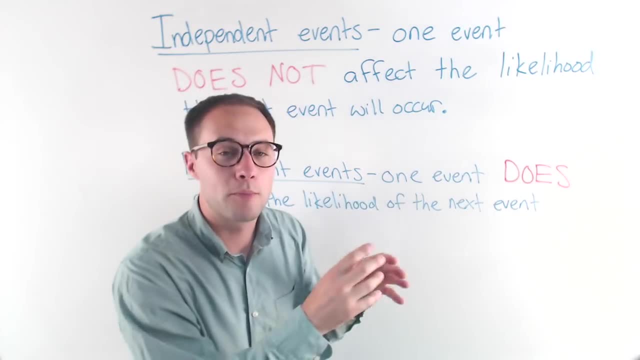 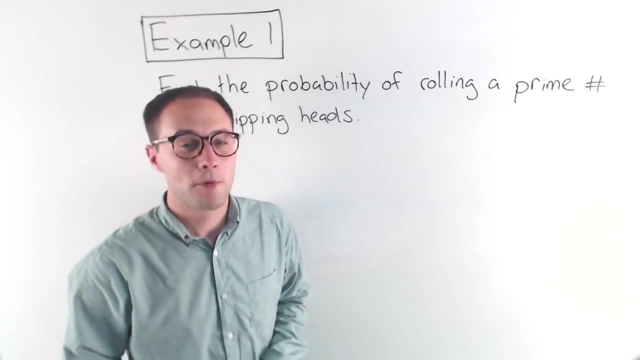 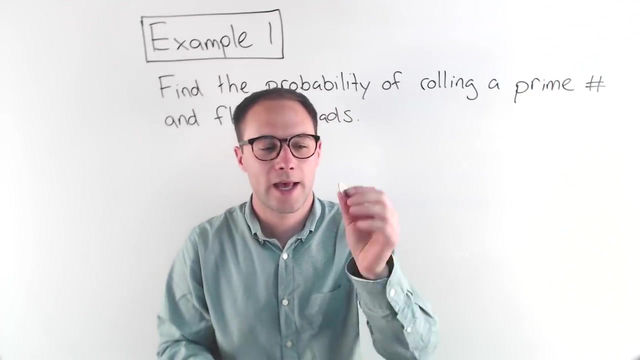 likelihood of the next event occurring. So the probability of the next event depends on what happens first. Let's look at an example. All right, example one: Find the probability of rolling a prime number and flipping heads. So we're talking about rolling a die and flipping heads on a coin. Now, if you think again, we're talking. 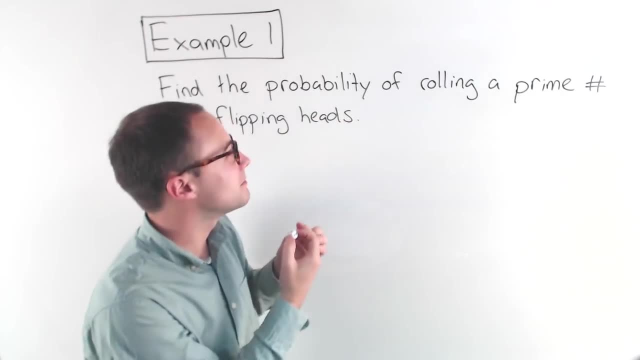 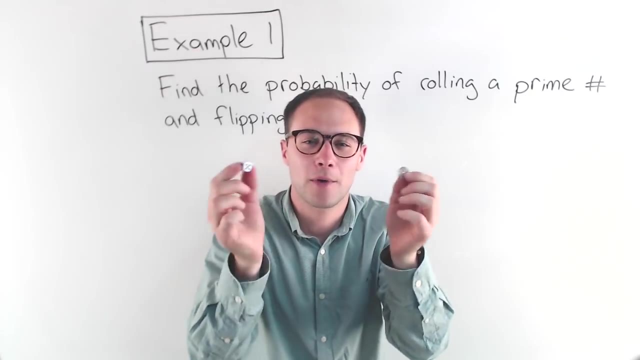 about independent or dependent events. what would this compound event be Independent or dependent? And hopefully you realize it's independent. Like we said, these don't care what the other did, They're independent of each other. So it's an independent event. Now for an independent. 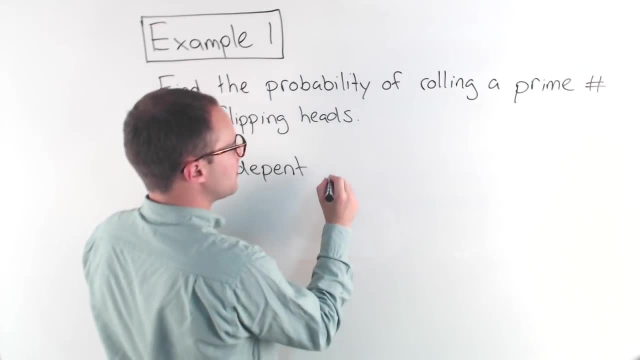 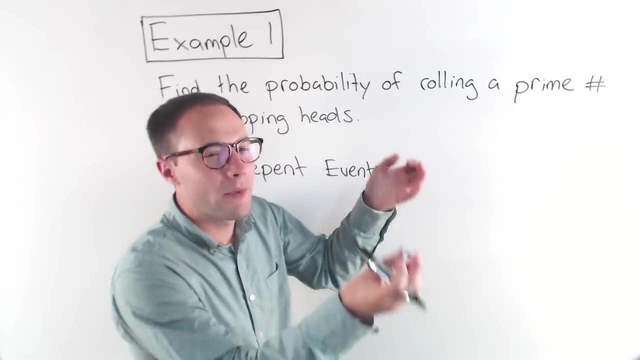 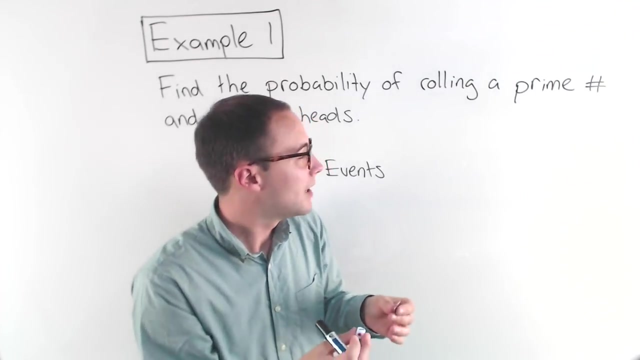 event. there's a formula we can use for finding the probability. Now you may have done before tree diagrams or tables to find all the possible outcomes and then you can find the probability that way, But that can take a lot of time. So instead we have a formula where the probability 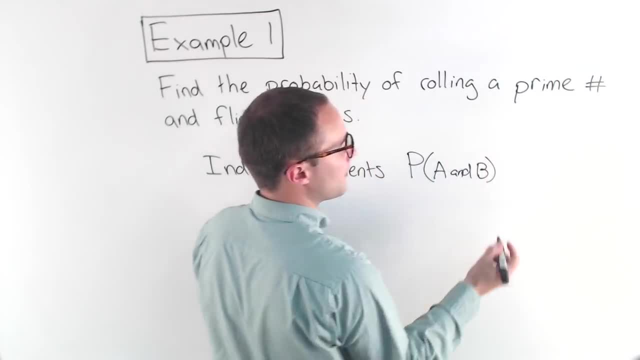 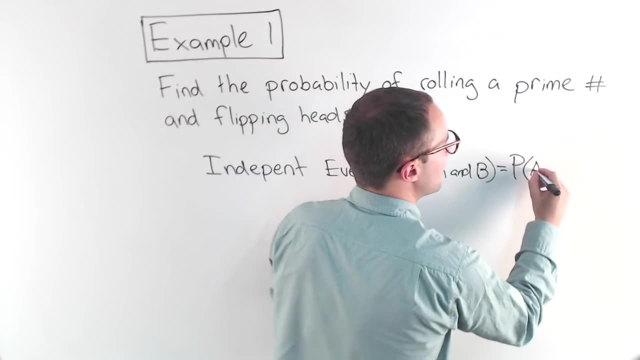 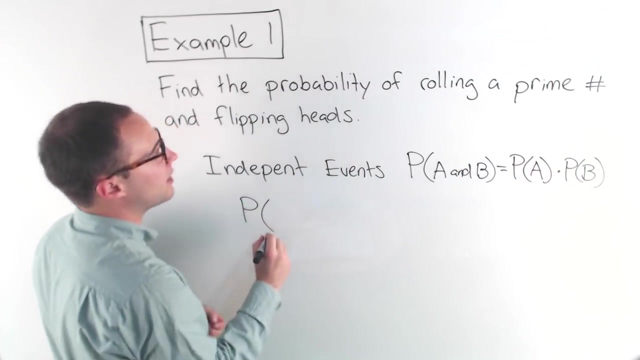 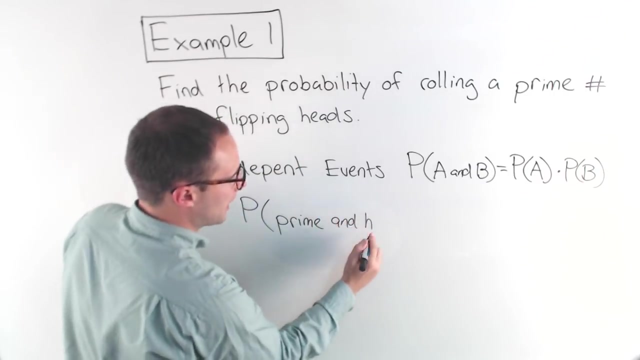 of A and B. that's equal to well, just the individual probabilities multiplied by each other. So probability of A times probability of B. Well, let's do that. So we're finding the probability of a prime number and heads. So I can just abbreviate. 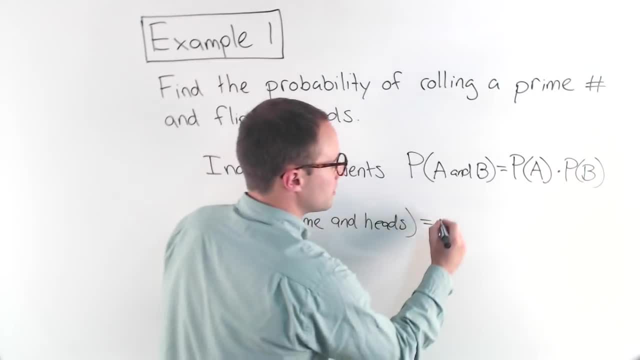 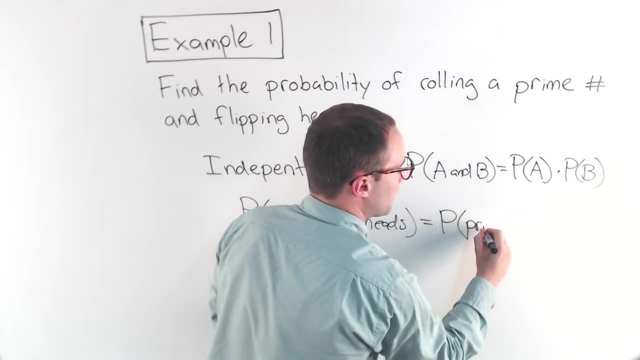 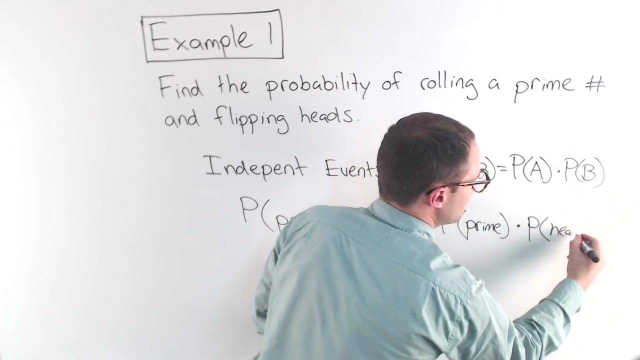 Probability of prime and heads is going to be equal to the probability of: well, what was A? What's that first event? A prime number. What's the probability of getting a prime number Times the probability of flipping heads? So, first, what is the probability of getting a prime number when you roll a die? 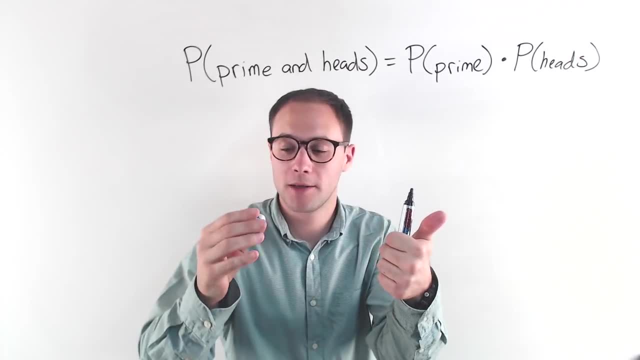 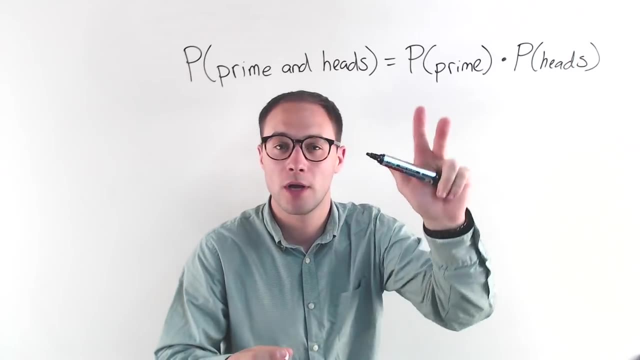 Well, 1 is not prime, 2 is prime, 3 is prime, 4, no, that's composite. 5, that is prime And 6 is composite. So 3 out of those 6 numbers are prime. 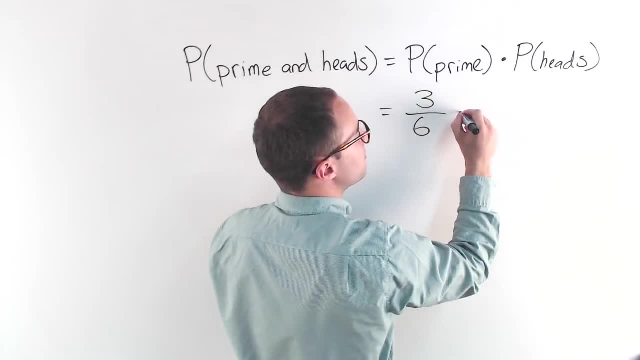 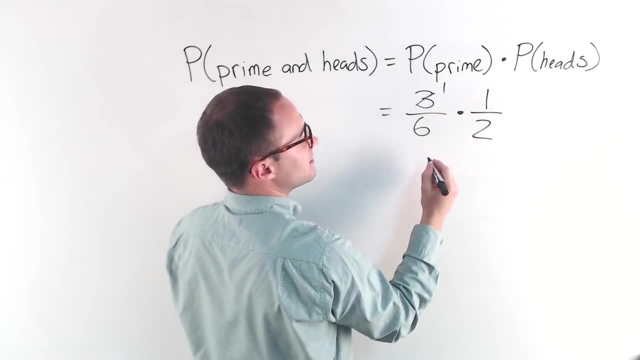 2, 3, and 5.. What is the probability of getting a heads? Well, 1 out of 2, right? We know that. So 3, 6 times 1 half. Well, I can make that simplified: 1 half and I get 1, 4.. Here's one to try on your own. 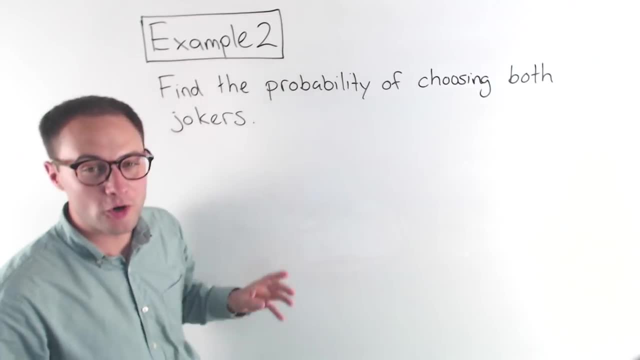 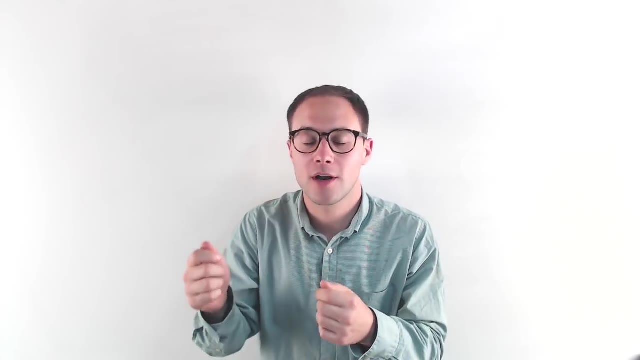 OK, example 2. Find the probability of choosing both jokers. Now, this is similar to what we did with Cal earlier. It's a very, very simple case. So this is an example of a joker and an adversaire. except with Cal, when he chose a joker, we put it back in the deck. this time, when we choose, 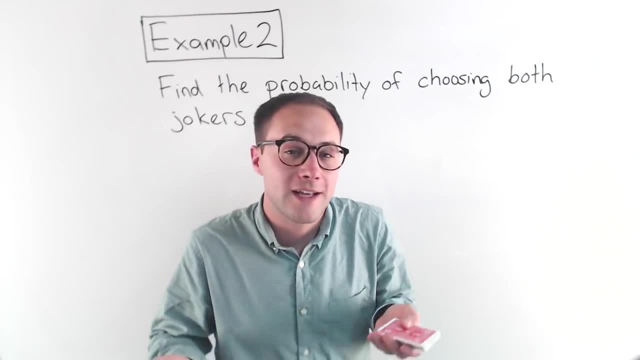 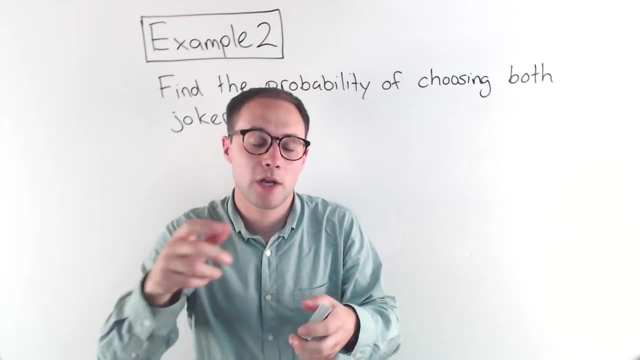 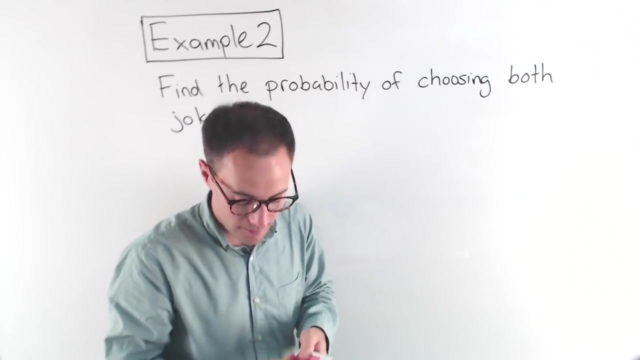 a joker, we're leaving it out first. is this independent or dependent? if you choose something and put it back, well then it doesn't affect the next time, but if you choose something and leave it out, it does, so you got to be careful with that. so this is a dependent event. let's go over first. 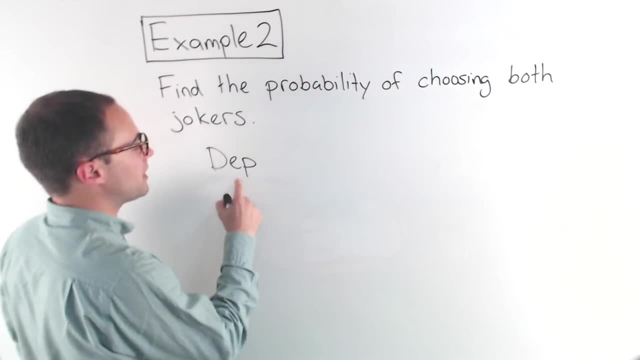 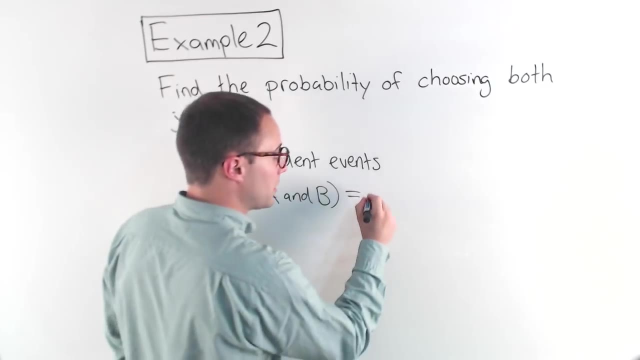 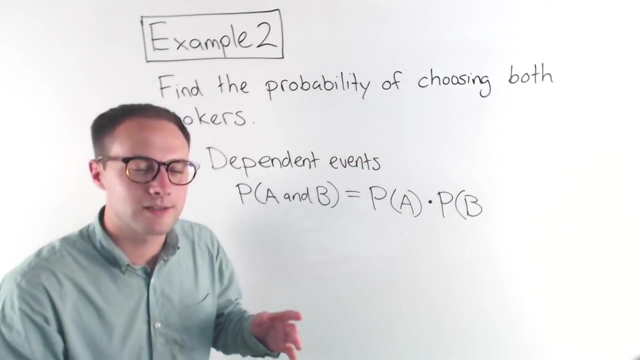 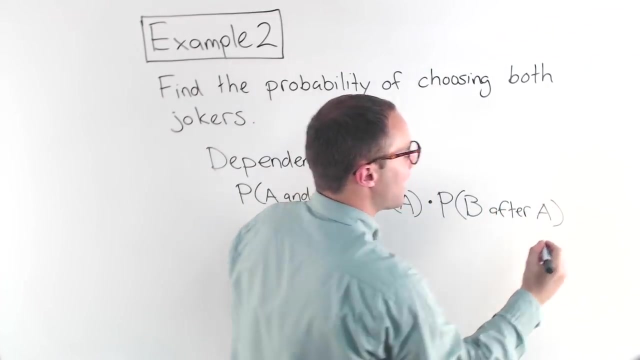 the formula for a deep ending event, probability of A and B is going to be equal to the probability of a. whatever's happening first times the probability of B. now, this is where it's a little different. the probability of getting B after a, after a, has already happened. well, first, 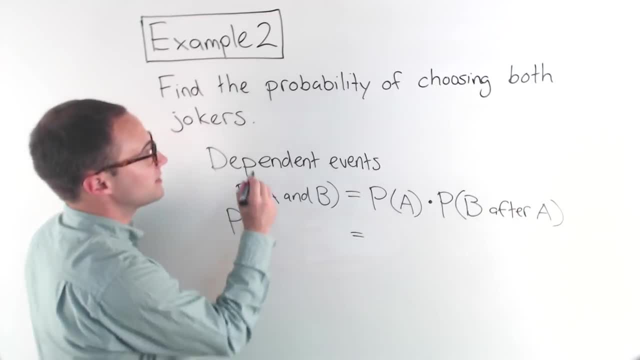 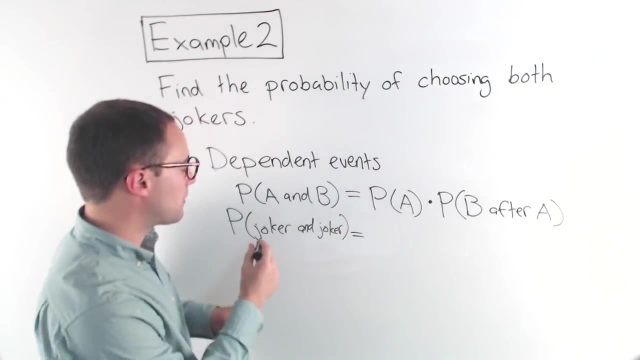 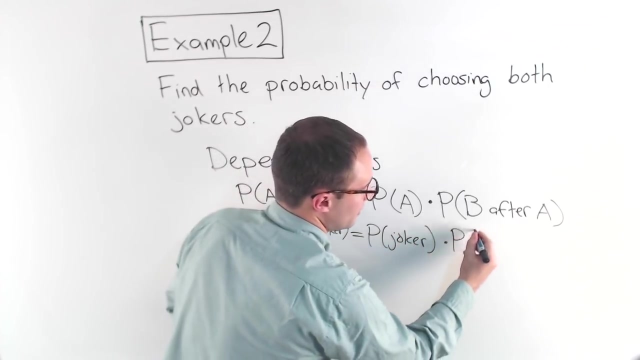 probably A and B. well, I'm doing probability of, in this case, a joker and another joker, right, We want both jokers. So probability of jokering a joker, so that's probability of getting a joker times probability of- and this is getting 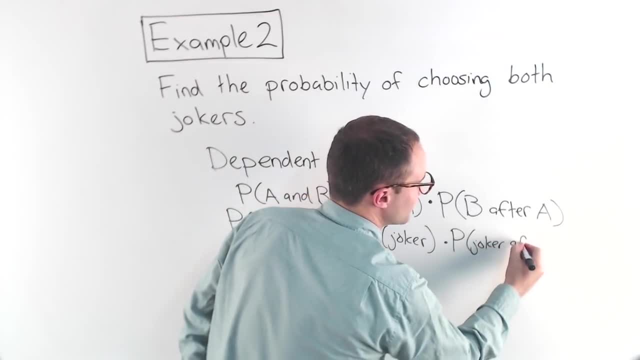 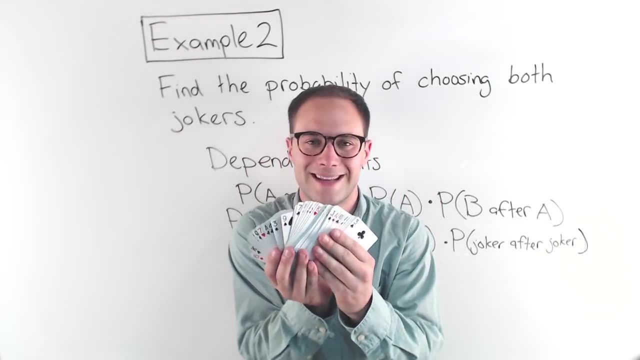 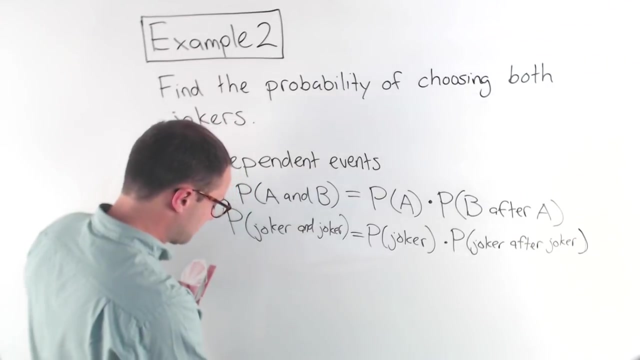 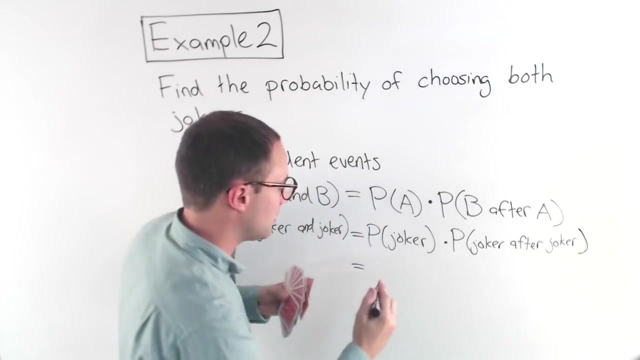 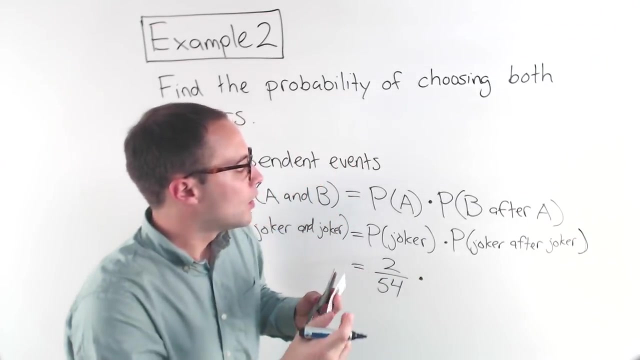 repetitive joker after a joker's already been chosen. Again, there's 52 normal cards in a deck. There are two jokers, So all together there are 54 cards. So the probability of choosing a joker the first time is two. there's two ways to get it out of 54 total cards. okay, Now what's the? 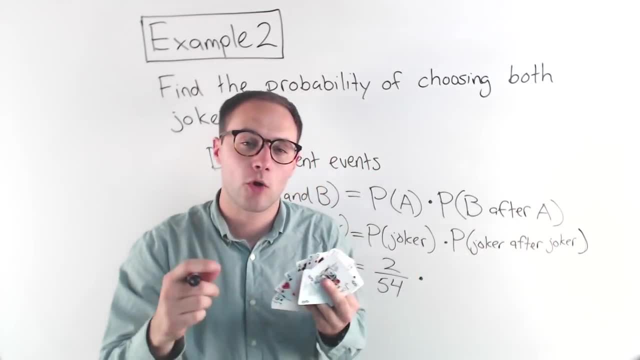 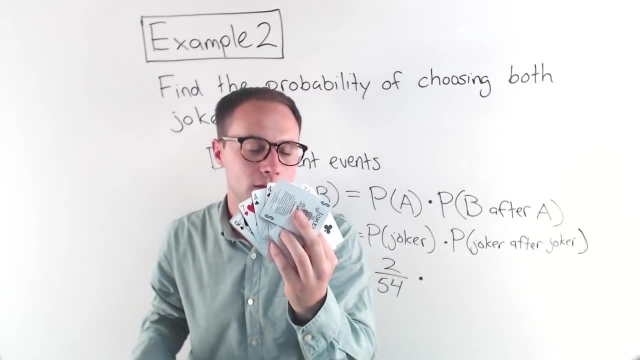 probability of getting a joker after a joker's already been chosen. Well, imagine that. So if we already chose that joker, now there's only one joker left. one way to get a joker, And right, we took a card away. So now, 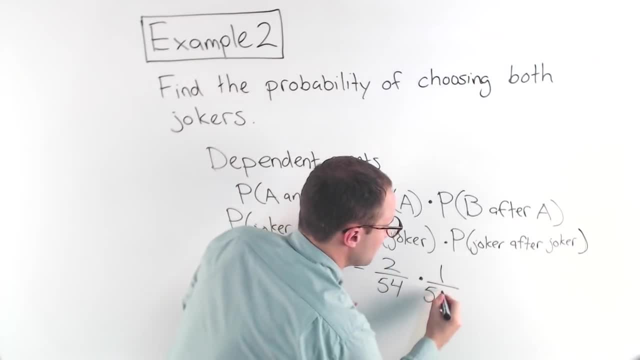 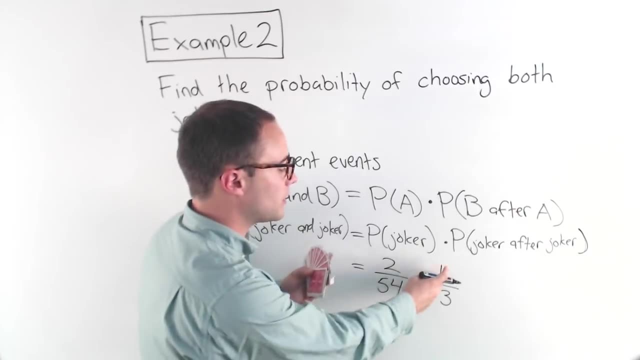 there's only 53, 53 cards total, So that's the probability of getting the next joker only one out of 53, because we assume we already chose one. okay, So now we can finish doing this, So I can. 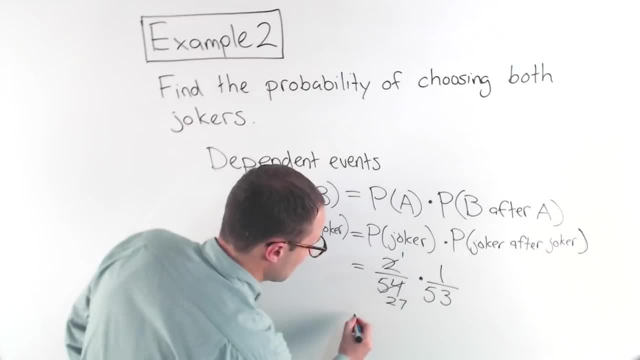 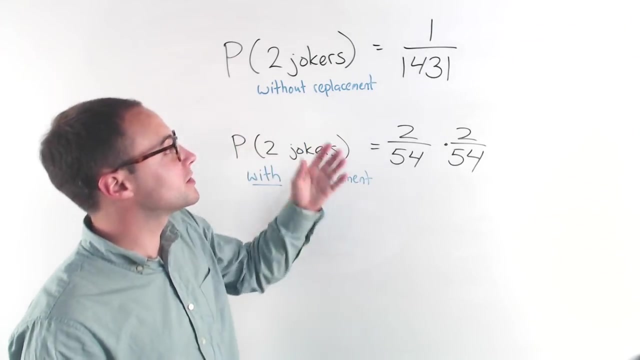 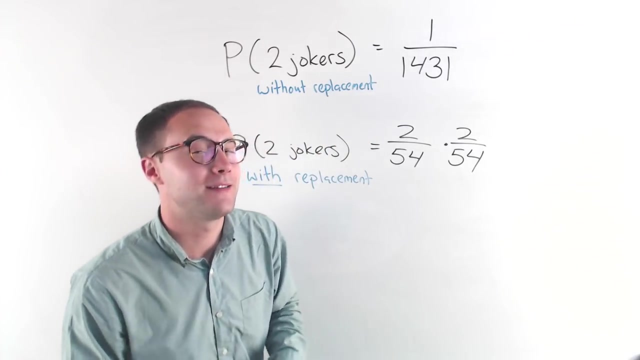 simplify that becomes one and 27.. One times one is one, 27 times 53, that is one out of 100, 1,431.. So probably getting two jokers without replacing, which is what we just talked about- one in 1,431, very, very difficult. But if you're wondering, 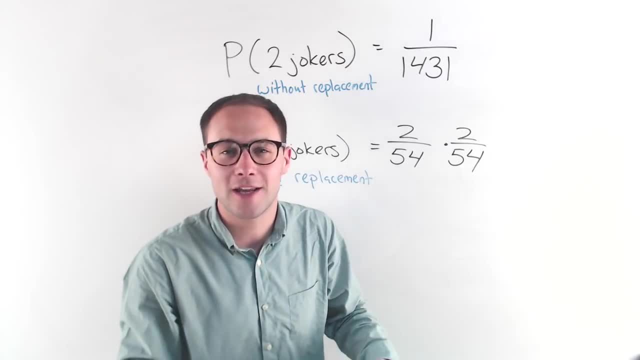 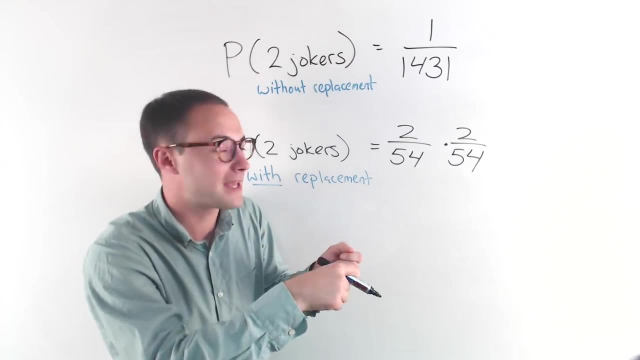 what Cal did earlier, right? Is he just very, very lucky? Well, probability of getting those two jokers right: A joker and then another joker with replacement, remember we put it back in. well, that's 2 out of 54. for that first joker, There's two. 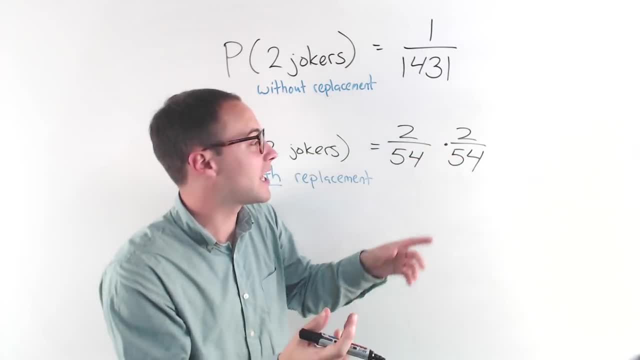 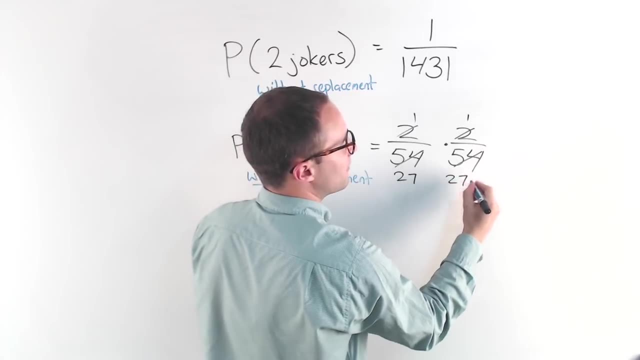 jokers 54 total. The next joker: it's still the same because we replaced it. That could simplify to 1 and 27.. Same thing here: 1 and 27,, which equals 1 and 729.. So 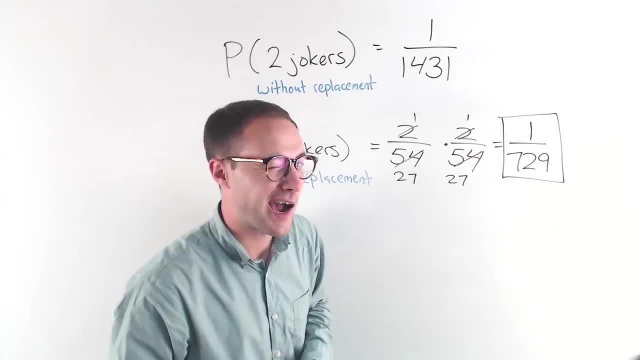 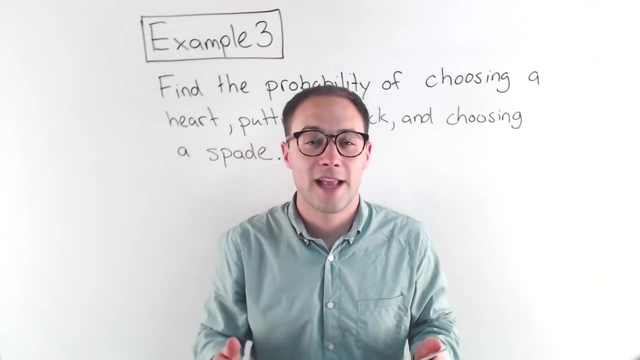 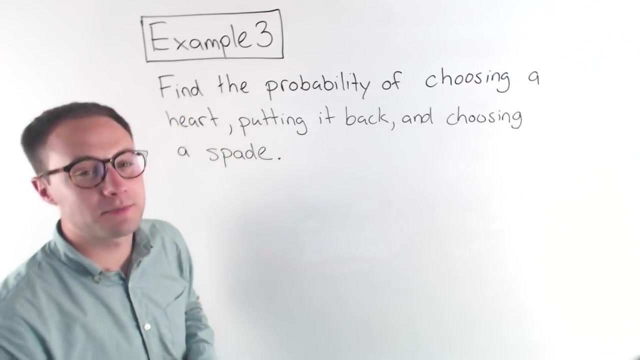 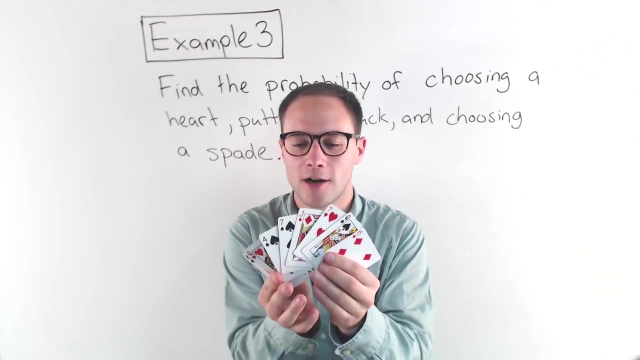 obviously Cal is very, very lucky. Okay, here's the last example, Example 3. Find the probability of choosing a heart, putting it back and then choosing a spade. So here are my cards. If you count them all up, you should notice there are. 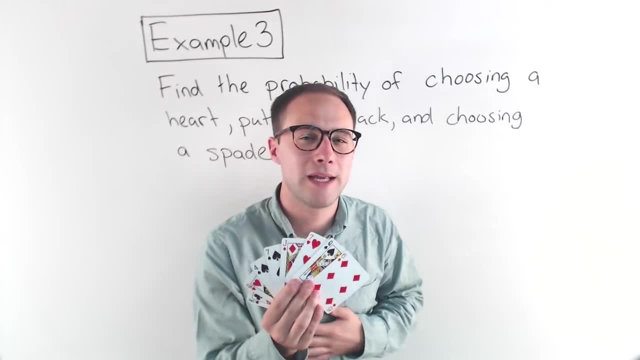 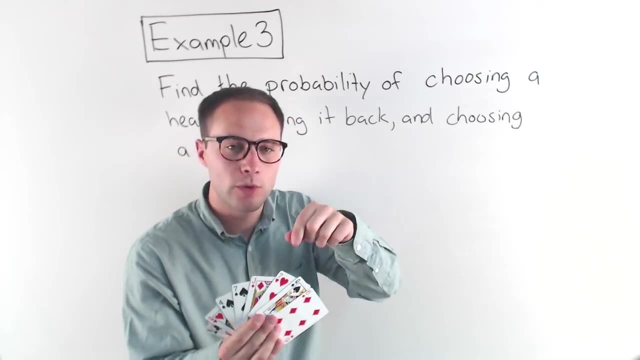 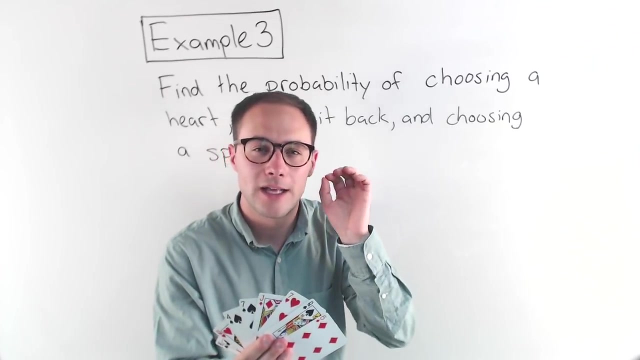 8. Now we gotta think first: is this gonna be dependent or independent? The key phrase here is that we put it back after we do the first, after we choose the first card. So that should tell you things aren't changing. It's gonna be. 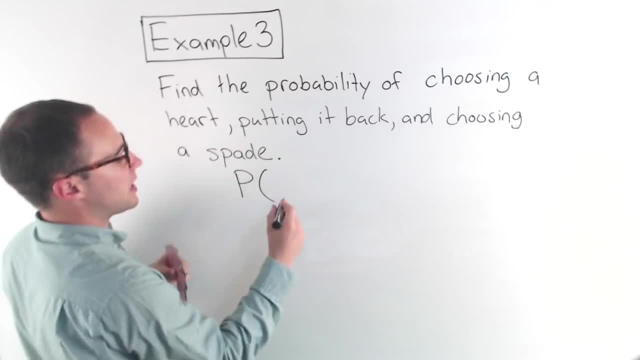 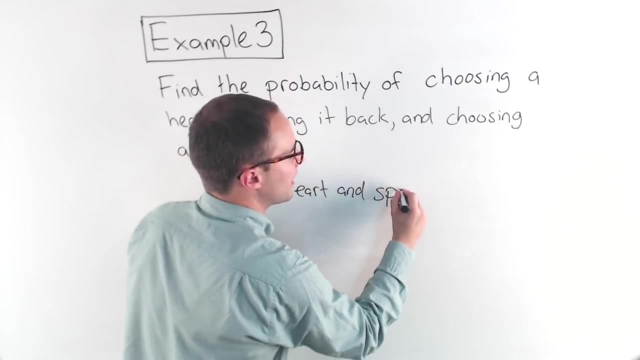 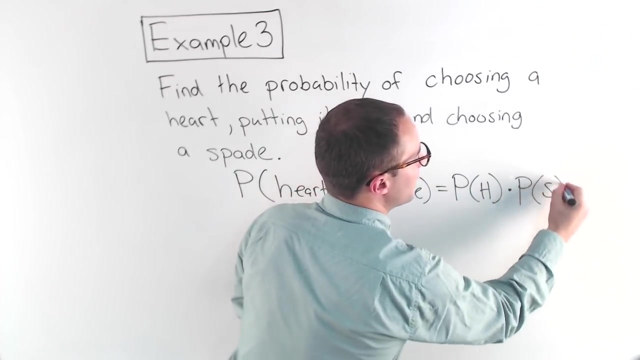 independent, The probability of choosing a heart, putting it back and then choosing a spade. So, heart and spade, That's just gonna be the probability of the heart times the probability of the spade. Well, what's the probability of choosing a heart? Well, how many hearts are there? 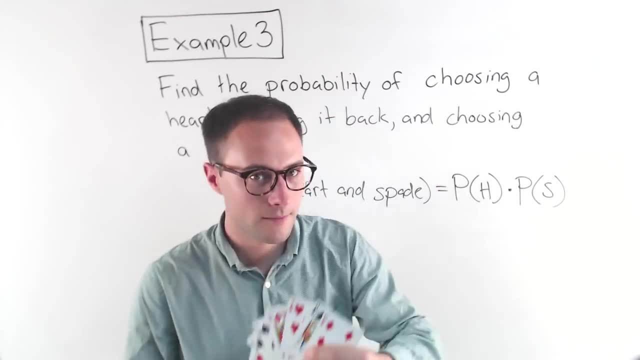 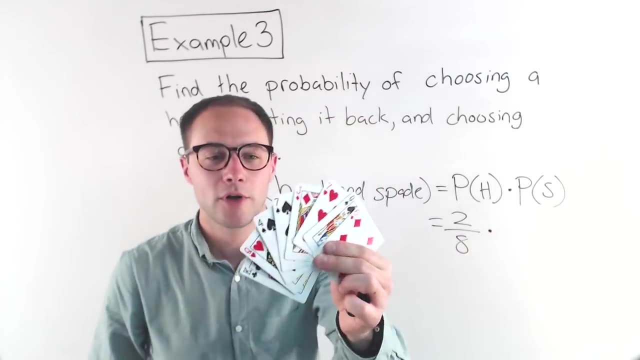 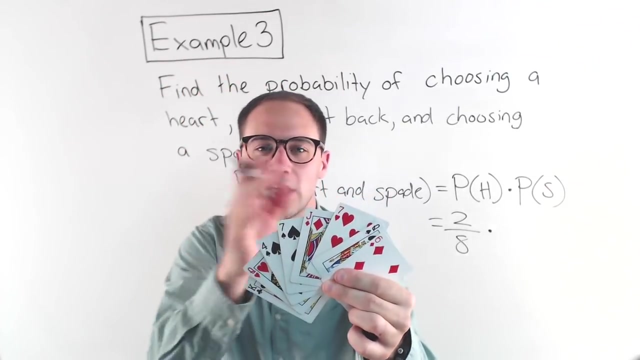 There are 1,, 2, right, The probability of a heart is 2 out of 8 total times the probability of a spade. So remember, if we choose a heart but we put it back, so things aren't changing, There's still 8 total.